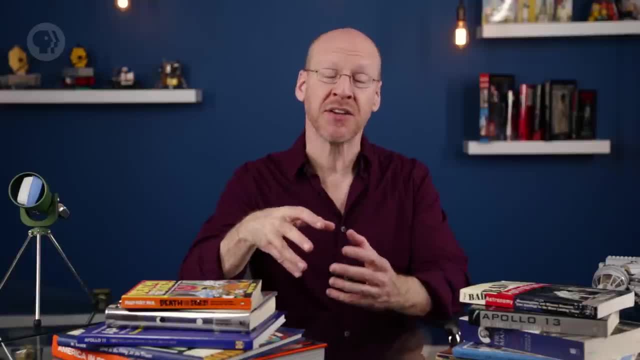 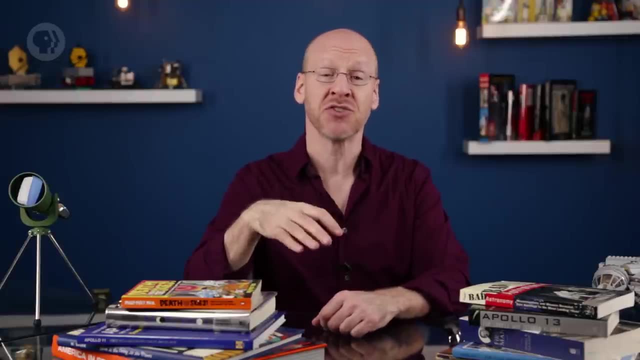 In science terms, mass tells us how much an object resists having its motion changed. An object with more mass is harder to get moving than an object with less mass, which is pretty obvious if you've ever tried pushing on a toy truck versus a real truck. But mass 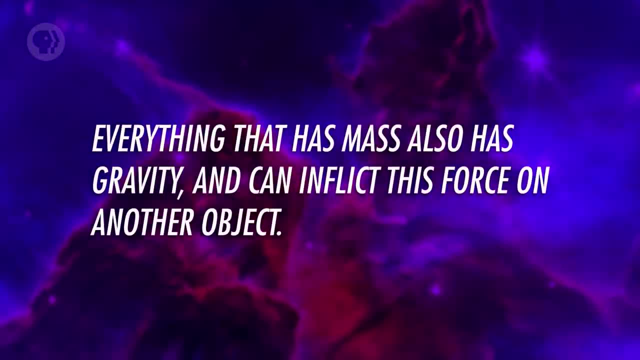 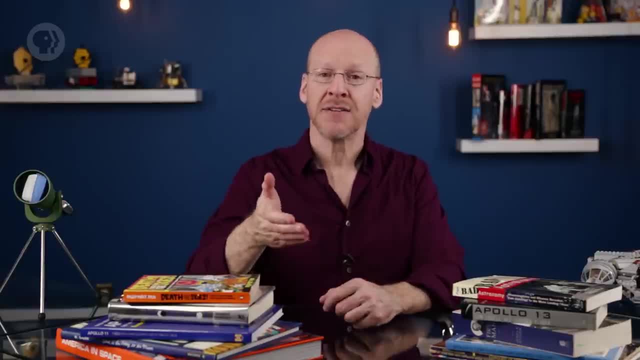 is also defined using gravity. Everything that has mass also has gravity and can inflict this force on another object. The amount of force you feel from the gravity of an object like a planet, depends on the three things: How much mass it has, how much mass you have and how far away you are from. it. In fact, distance dominates here. The force of gravity weakens with the square of the distance. Double your distance from an object and the force of gravity drops by 2 times 2 equals 4 times. Go 10 times farther away and the force drops by 10 times 10- equals. 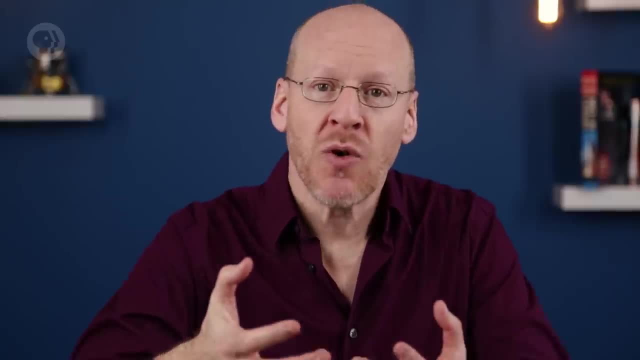 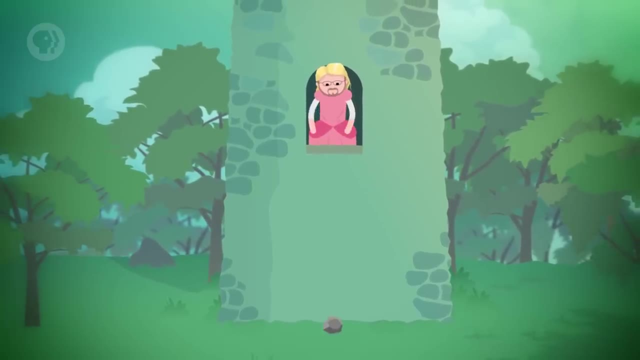 100 times Gravity is also attractive. It can only draw things in, not repel them. But how it attracts things is where it gets fun. If I hold up a rock and let go of it, it falls to the ground. What might be hard to see is: 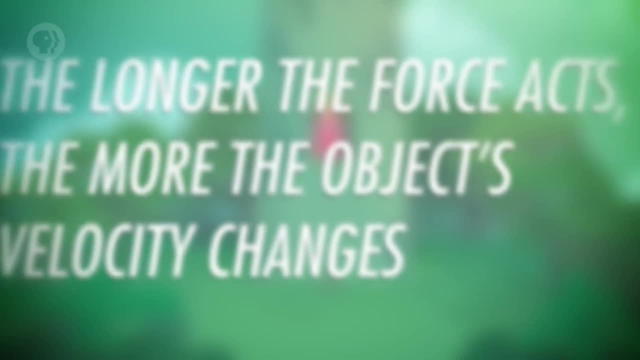 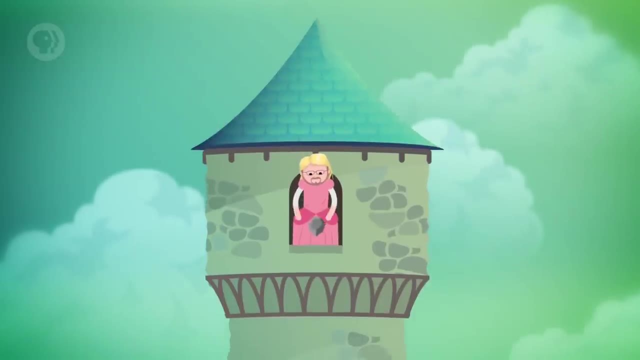 that it gets faster the longer it drops. Forces accelerate objects, so the longer the force acts, the more the object's velocity changes, in this case getting faster. If I drop a rock from higher up, it'll move faster when it hits the ground. 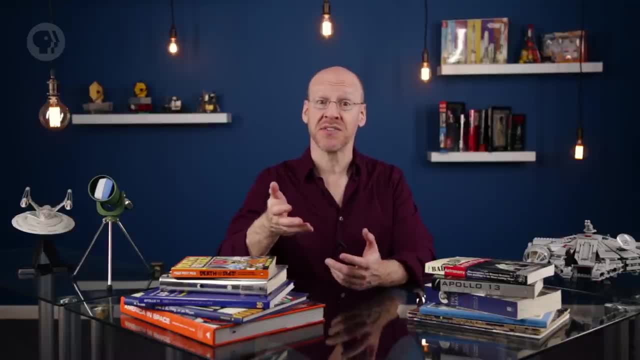 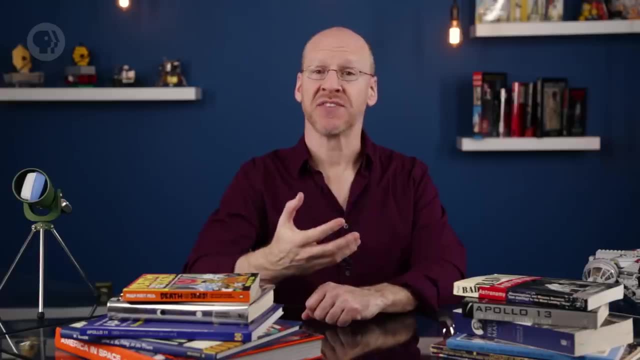 Other forces act on moving objects as well, like friction and air resistance, counteracting gravity, making this acceleration hard to see. But in space the force of gravity becomes very clear: Two objects that have mass will attract each other If there are no other forces acting. 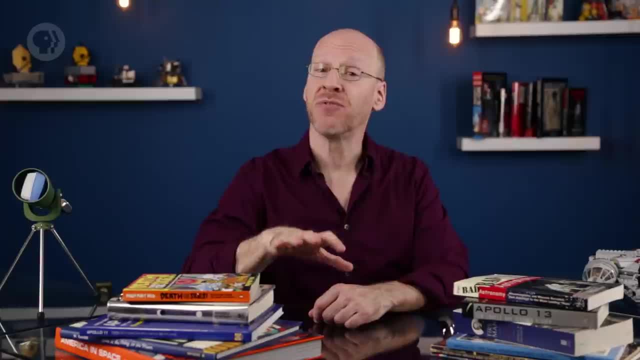 on them, they'll accelerate toward each other until they meet. Remember, though, that the force of gravity depends on those masses. If one is really massive and the other not so much, then, in more practical terms, the massive one will pull in the less. 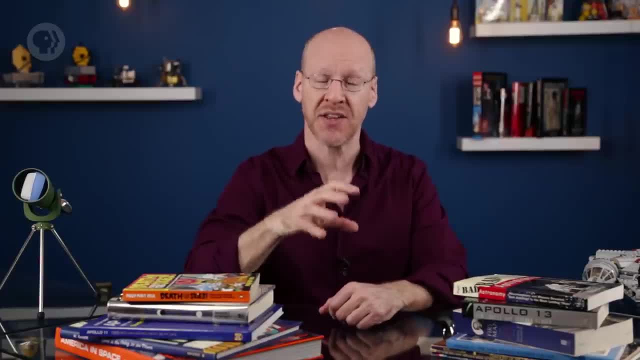 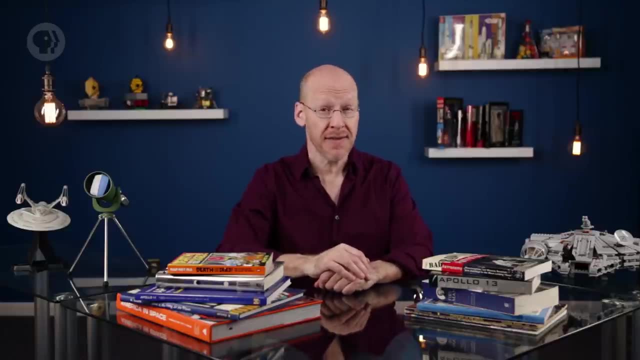 massive one. The more massive one does move, but much less than the other one. When objects are free to move under the effects of gravity, we say they are in orbit. The simplest kind of orbit may not be what you think. It's actually just a line When you 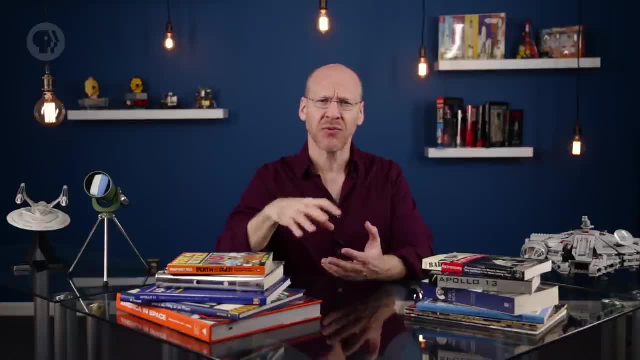 drop a rock, it's very briefly in orbit, Ignoring things like the Earth's rotation, which adds a bit of sideways motion. it's close enough to say the rock just falls straight down and is stopped because the Earth itself gets in the way. 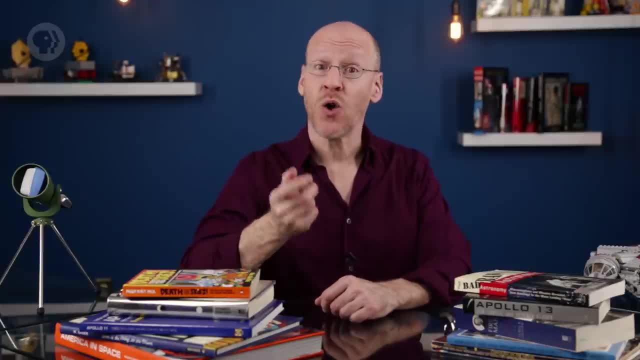 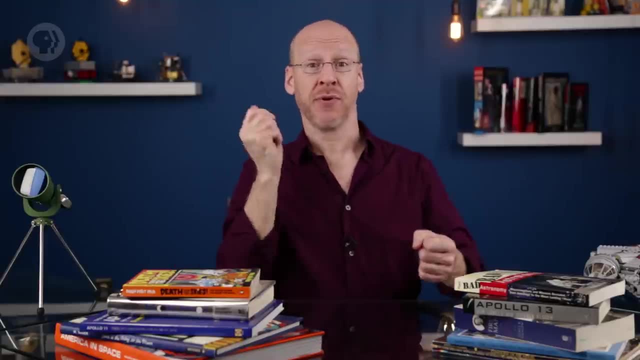 That's not a terribly interesting orbit. So what if, instead of dropping the rock, we throw it? That gives it a little bit of sideways motion. so instead of hitting the ground at my feet, it hits a bit farther away. If I throw it harder, it moves horizontally even more before it hits. 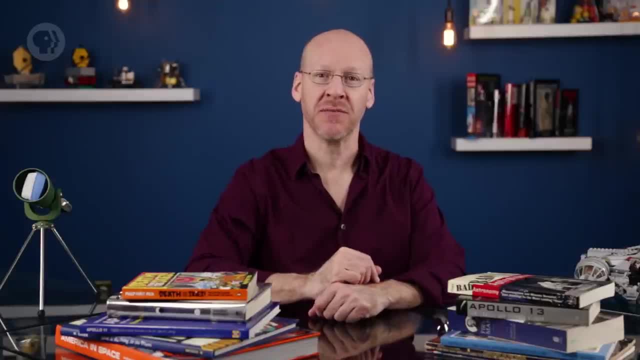 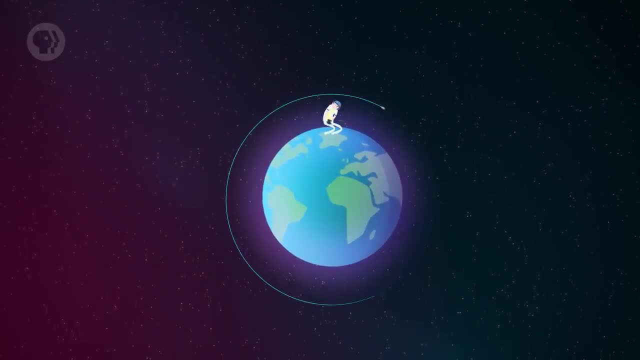 What if I throw it really hard? This is where Newton's genius comes in. He realized that if you throw the ball hard enough, sideways it will fall at the exact same speed. At the exact same rate, the Earth would curve away underneath it. As Douglas Adams said in Hitchhiker's Guide to the Galaxy, flying is just falling and missing the ground. It turns out that's exactly what orbiting is too: A rock thrown hard enough sideways will fall toward the Earth, but always miss it going. 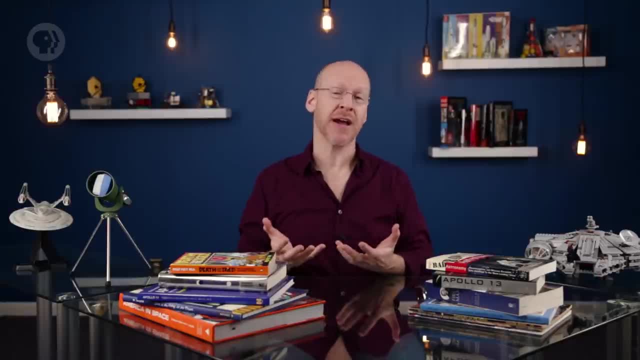 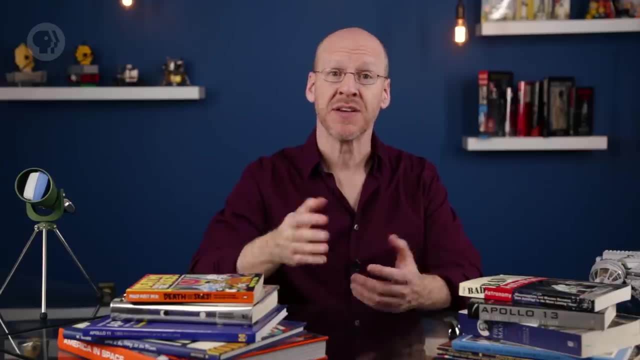 instead into a circular path around it, guided only by gravity. It'll orbit the Earth in a circle, taking about 90 minutes to go around the planet. once Circles are simple orbits, The speed at which the orbiting satellite travels depends on. the mass of the object it's orbiting and its distance from it. The farther it is, the weaker gravity is, so it doesn't have to travel as quickly to maintain the orbit. Roughly 400 years ago, the astronomer Johannes Kepler realized that there can be other shapes. 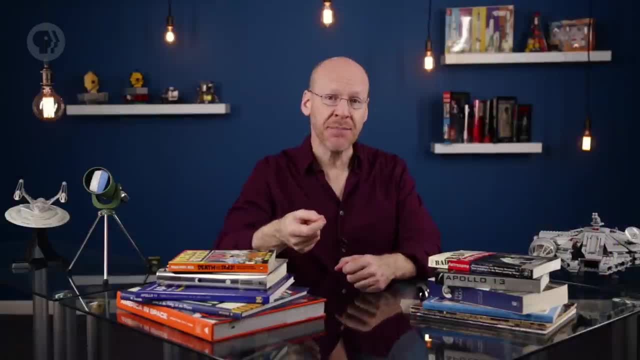 of orbits as well. He discovered that planets orbit the Sun on ellipses when previously it was thought they orbited in perfect circles. An elliptical orbit happens when you throw the rock sideways even harder than it takes for a circular orbit. It goes up higher on one end of the orbit than on the other. In 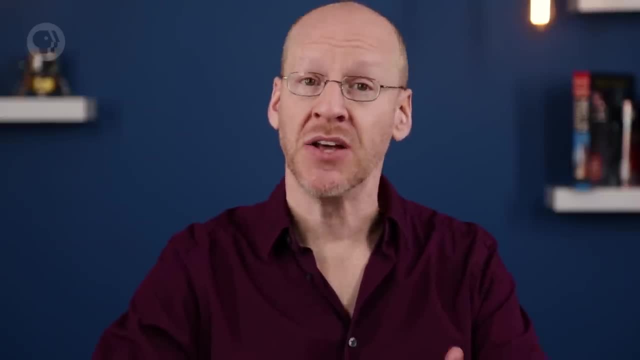 fact, the harder you throw the rock, the more it will go up. The longer you throw the rock, the more elongated the orbit gets. An orbit like this is still closed, That is, the orbit repeats itself and the rock is still bound to the Earth by. 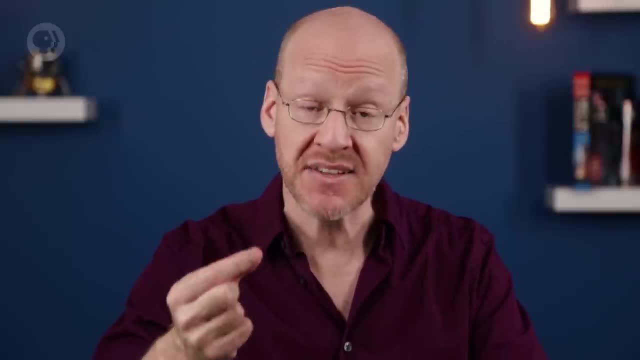 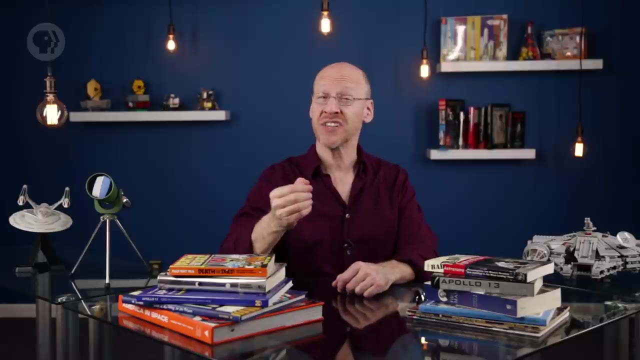 gravity. At some point, though, if you throw the rock hard enough, an amazing thing happens: It can escape. Remember: gravity gets weaker with distance. If you throw a rock hard enough, while gravity can slow it down, the gravity gets weaker the farther away the rock is. If the rock 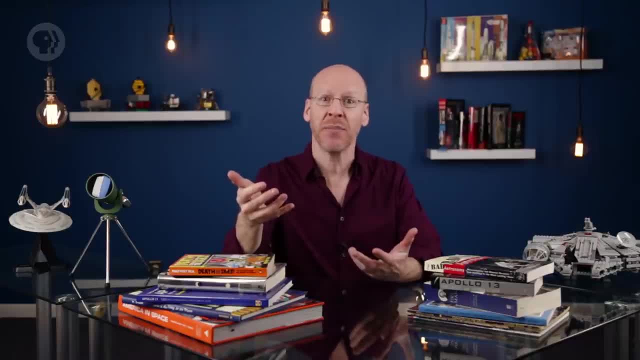 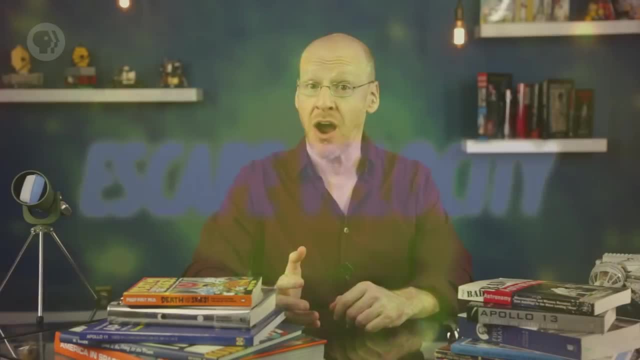 has enough velocity, gravity weakens too quickly to stop it. The rock can escape, moving away forever. What is the escape velocity? The escape velocity of an object, like a planet or star, depends on how much mass it has and how big it is. For the Earth, that turns out to be about 11 kilometers per second. For 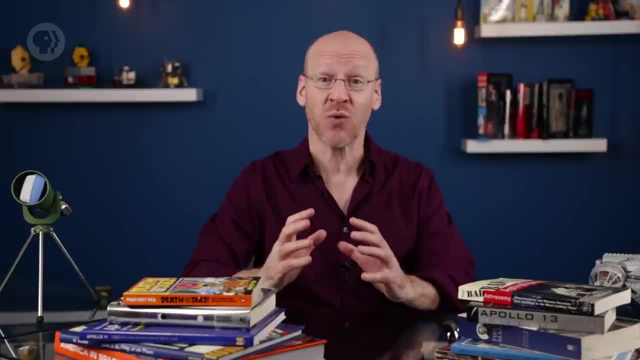 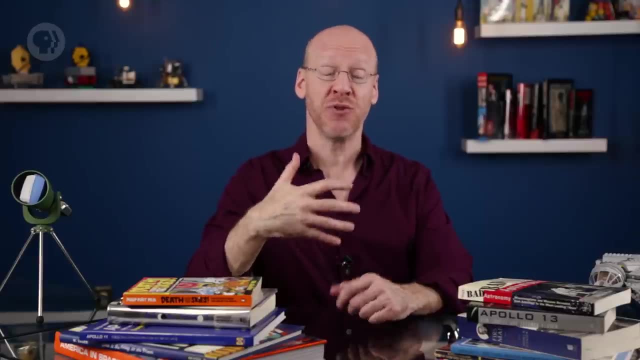 Jupiter it's about 58 kilometers per second, And for the Sun it's a whopping 600 kilometers per second. Whatever the particular escape velocity for your cosmic location is, if you fling a rock away from it faster than that, I hope you kissed it goodbye first, because it ain't. coming back, One way to think of it is that the rock is always slowing, getting ever closer to the Earth. It's closer to stopping, but it never actually stops. If it could travel infinitely far away it would stop, but that's kind of a long trip. 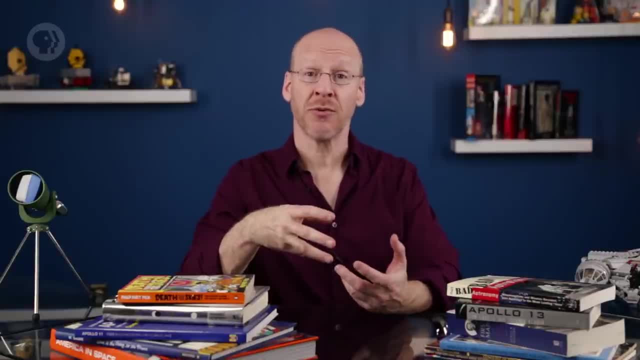 This works in reverse too. If I go way, far away from the Earth and drop a rock, it'll accelerate. When it hits the planet it'll be moving at escape velocity- that same 11 kilometers per second. And if I give it a little sideways kick, it'll miss the Earth. but still pass us at escape velocity. An escape orbit is open, it doesn't come back and is shaped like a parabola. What if you throw the rock even harder than that? The rock doesn't come back and moves away even faster. The orbit is now a hyperbola. 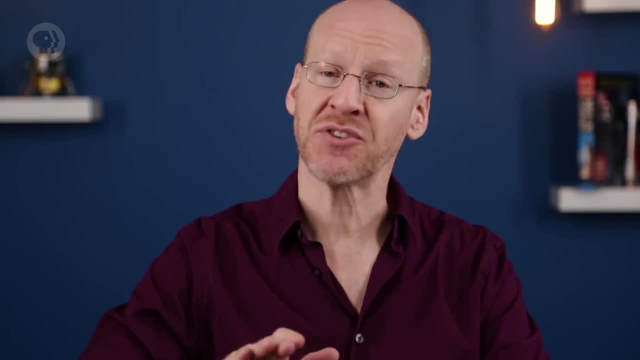 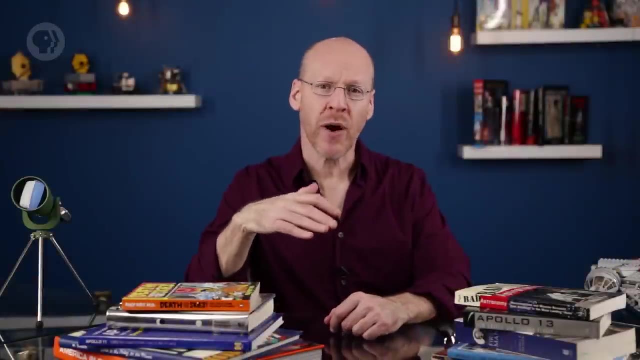 which is similar to a parabola, but is even more open. The rock never stops, even at infinity. It just keeps moving up. Like all forces, gravity gets weaker with distance, But its force never quite drops to zero. It just gets smaller and smaller as you get farther and farther away. 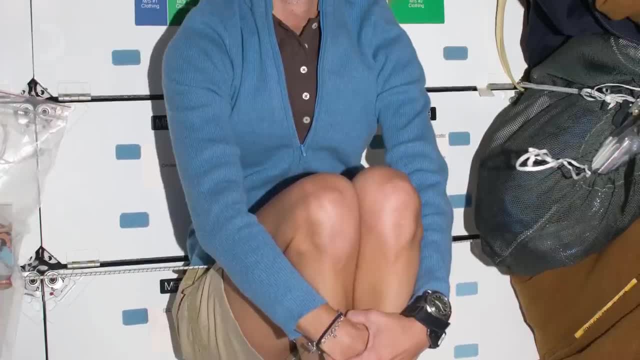 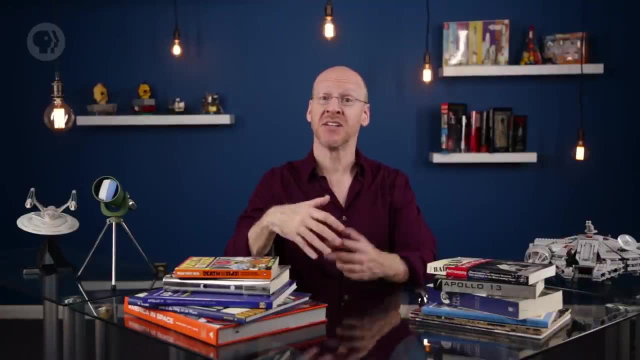 So why then are astronauts on the space station weightless? Gravity is still pulling on the astronauts. In fact, at the height of the station, Earth's gravity has only decreased by a little bit. If you look at the Earth's surface, it's still about 90% as strong as it is on the Earth's surface. If they were in a tower 320 kilometers high, they'd weigh 90% of what they'd do on the Earth's surface. But the big difference is that the astronauts are in orbit falling around the Earth. Weight is actually not just the force of gravity on a mass, but how hard a surface pushes back. 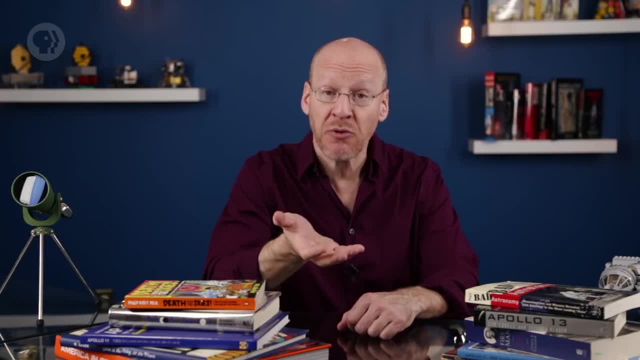 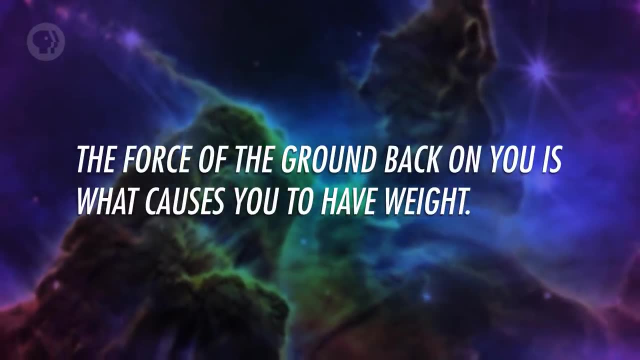 on that mass. For example, when you stand on the ground, the ground pushes back, otherwise you'd fall through. The force of the ground back on you is what causes you to have weight. It's under 10 centimeters. It's getting closer than you think, So what if you're? 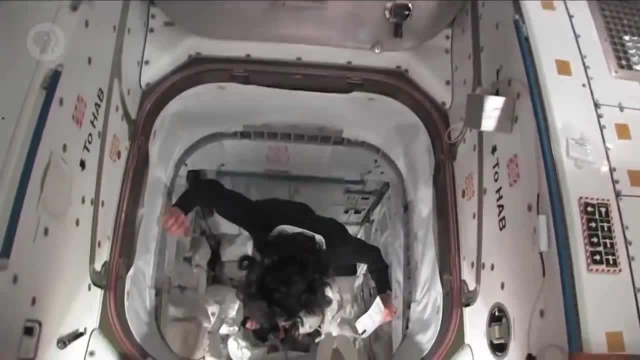 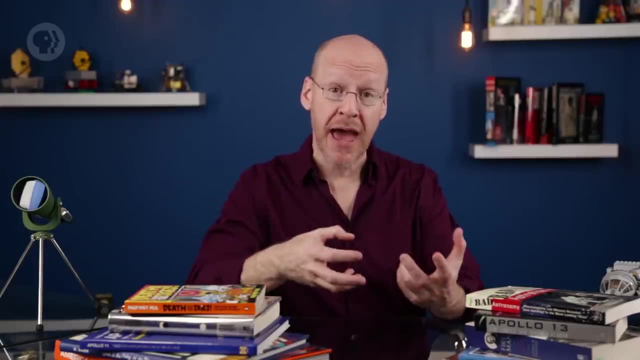 all, there's nothing pushing back. You're falling freely, and so you have no weight. NASA likes to call this condition microgravity, since there are subtle forces acting on you. This actually highlights the difference between mass and weight In space. you have the same. mass, as you do on Earth, but no weight. If another astronaut pushed on you they'd have to exert a force, but if you stood on a scale in space it wouldn't register or anything. Space is weird, Well compared to Earth. 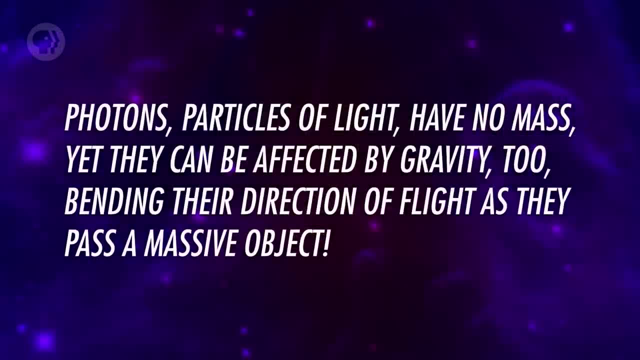 One more thing, and this is truly weird. Photons, particles of light, have no mass, yet they can be affected by gravity too, bending their direction of flight as they pass a massive object. It turns out gravity can actually warp space. Light travels along the fabric. 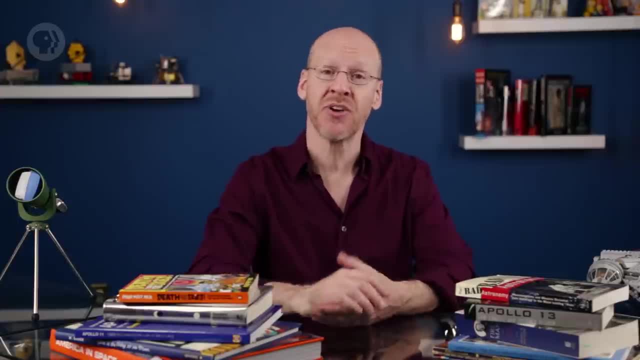 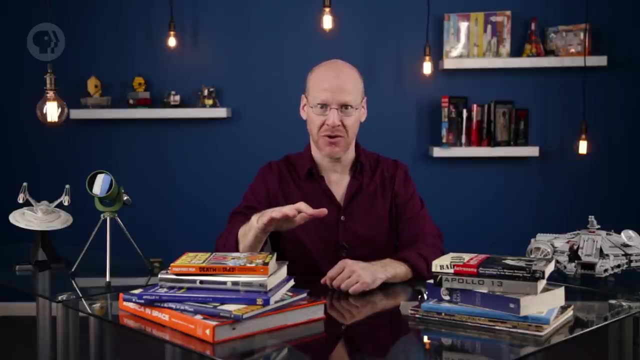 of space like a truck on the road, and if the road curves so does the truck. I know this is an odd concept and we'll be dealing with it later in more detail. when we push escape velocity to its limits with black holes, 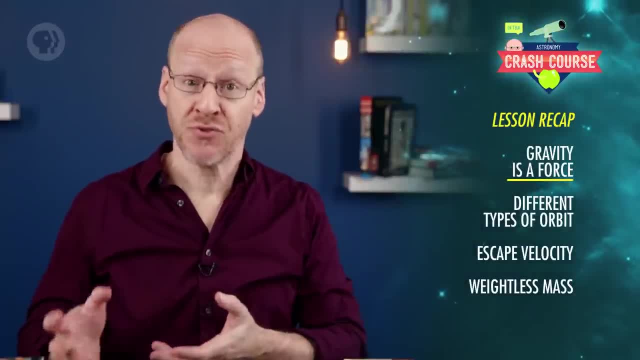 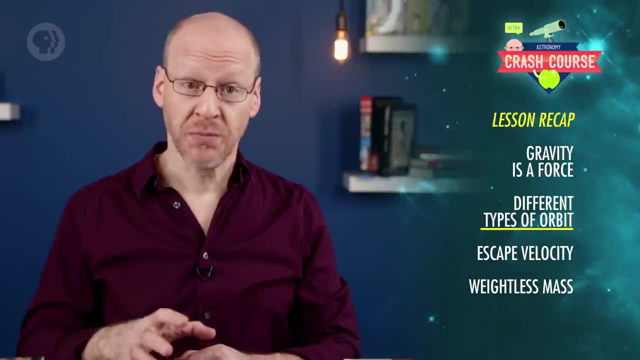 Today you learned that gravity is a force and everything with mass is a force. Space has gravity. Gravity accelerates objects with mass, changing their speed and or direction. An object moving along a path controlled by gravity is said to be in orbit, and there. 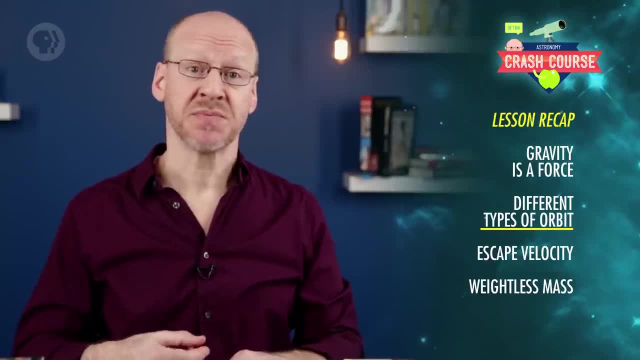 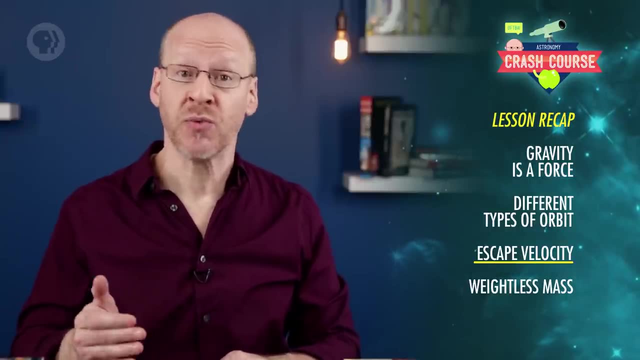 are many different kinds: Straight lines, circles, ellipses, parabolae and hyperbolae. You can't ever escape gravity, but if you travel faster than escape velocity for an object, you'll get away from it without falling back. And if you're in orbit in 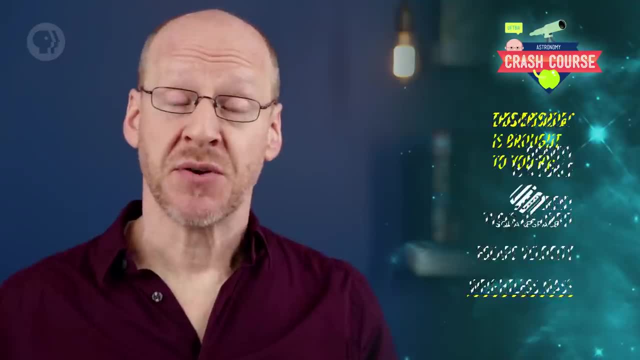 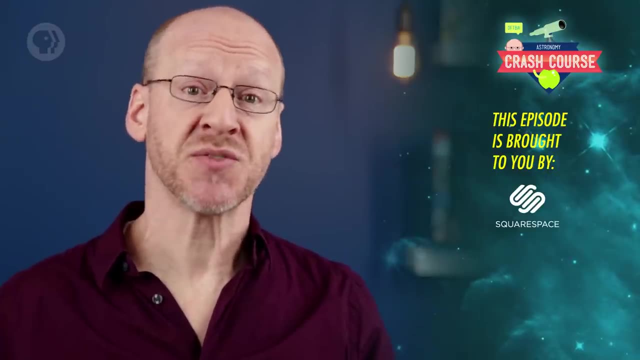 free fall. you have no weight, but you still have mass. This episode is brought to you by Squarespace. The latest version of their platform, which is Squarespace 7, has a completely redesigned interface. integrations with Getty Images.